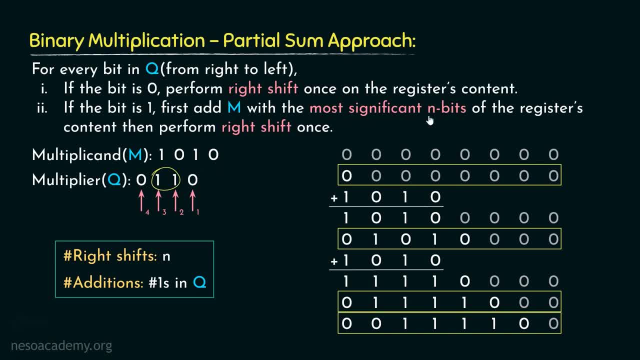 that is the entire multiplicand, that too, with the most significant n bits of the register content, and then perform the right shift. So basically, in the entire process, the number of shifts is n, where n denotes the number of bits in the multiplier, because either we come across the 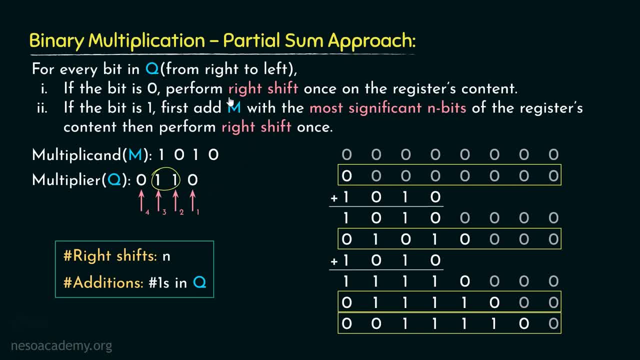 bit 0 or we come across the bit 1, we are going to perform the right shift once. And now, coming to the number of additions, that depends on number of ones in Q, Like in this particular case, we had to perform the addition twice because there were two ones in the multiplier. 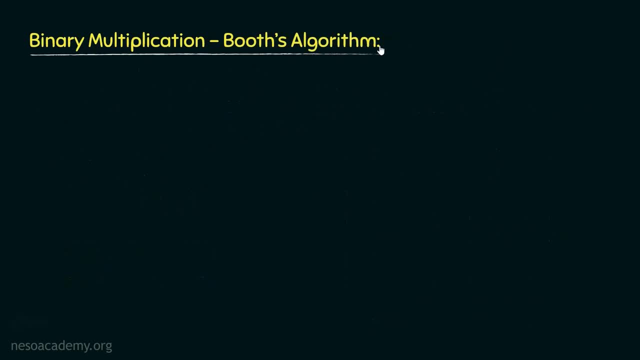 In today's session, we are about to observe how Booth's algorithm can increase the efficiency of the multiplication process with respect to the partial sum approach. Now, using Booth's algorithm, we can multiply two sine binary numbers in two's complement notation, And this algorithm was 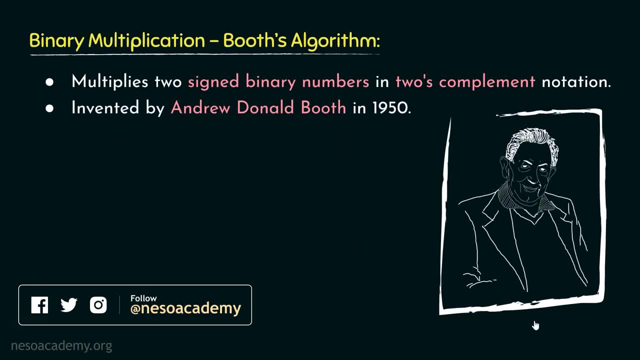 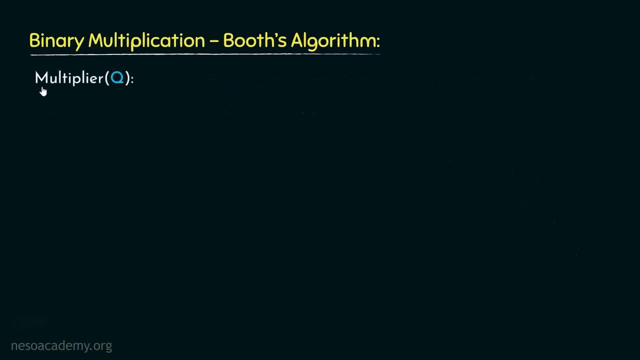 invented by Andrew Donald Booth in 1950 during his research on crystallography. Let's now dive into the concept of Booth's algorithm. Say we have a multiplier Q, which happens to be a sequence of ones having some leading and succeeding zeros. Now generally. 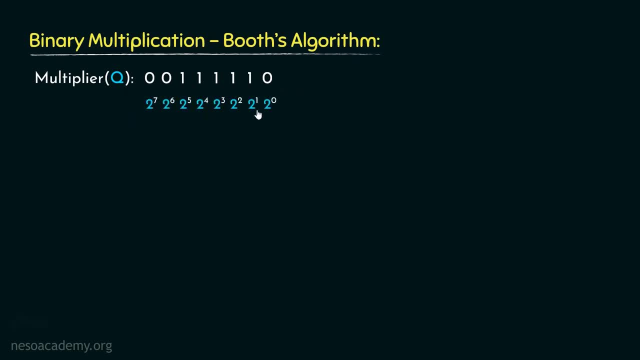 when we decode this into decimal, we use the place values, and thereafter we select the place values. which has ones in them, don't we So? this one is 2 raised to the power 5 or 32.. This one is 2 raised to the power 4 or 16.. Here we have 2 cubed, that is 8.. Then again we have 2 squared. 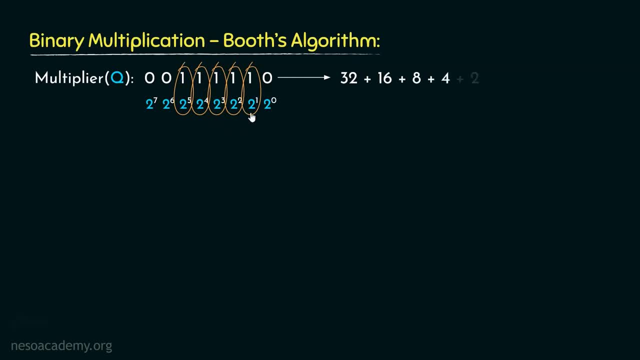 that is 4.. And finally, we have 2 raised to the power, 1.. 1,, that is 2.. Now, adding all these, we obtain the result 62.. Now, this is one way of decoding, but we can do one better. Observe the bit sequence. This is the first one, while we 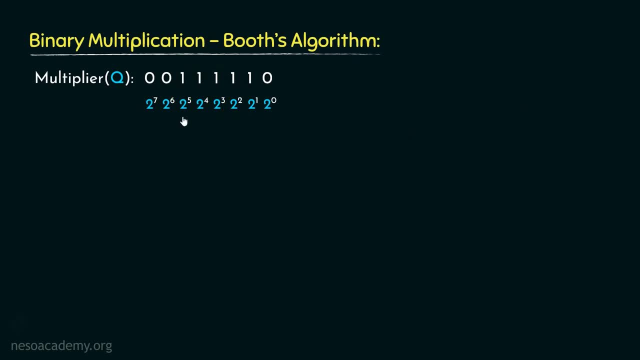 traverse the sequence from left to right. Now observe its place value. It is 2 raised to the power 5.. Now, instead of taking this place value, we are going to take the place value of the previous one. Or in other words, we can say we will take the place value 2 raised to the power. 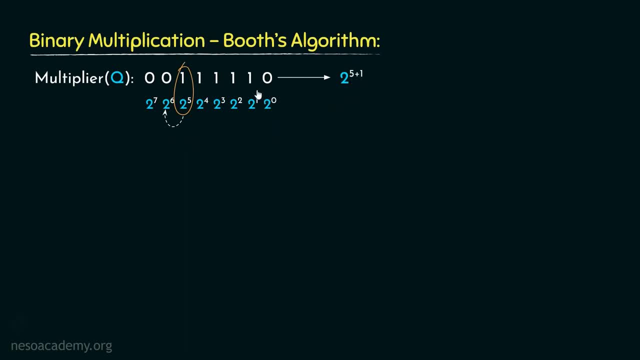 5 and we will add 1 to it. Now observe the place value of the last one in the sequence: It is 2 raised to the power 1.. Now if from this, that is 2 raised to the power 5 plus 1,. 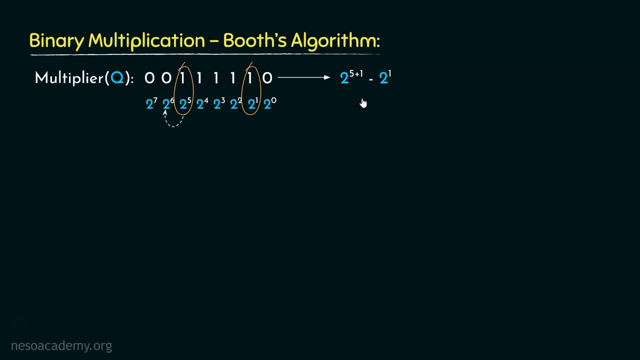 we subtract 2 raised to the power 1, let's see what happens Now. 2 raised to the power 5 plus 1 is 2 raised to the power 6 or 64. And 2 raised to the power 1 will simply give us 2.. So 64 minus. 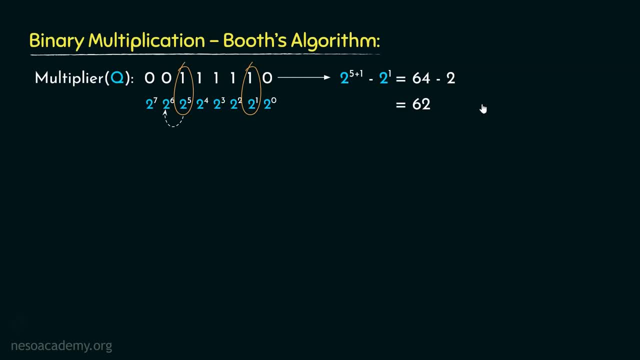 2 is 62. Interesting, isn't it? Now, this particular concept works for a sequence like this as well. Let me illustrate. We will first take the place values. Now observe the first sequence of ones. The place values of these are: 2 raised to the power 6. 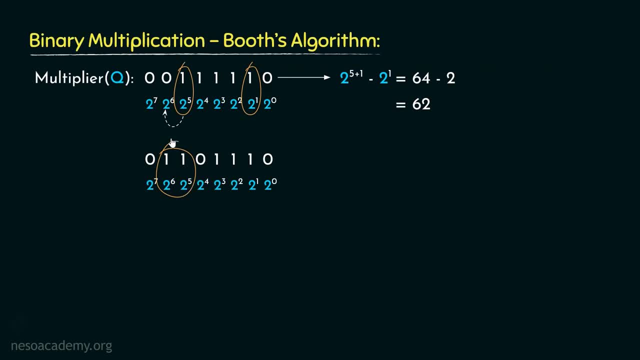 and 2 raised to the power 5.. Now, the decimal value which we can retrieve from these two bits can be obtained by stating: 2 raised to the power 7 minus 2 raised to the power 5.. Now, 2 raised to the power 7 is nothing but 2 raised to the power, 6 plus 1,. right Now, coming to the 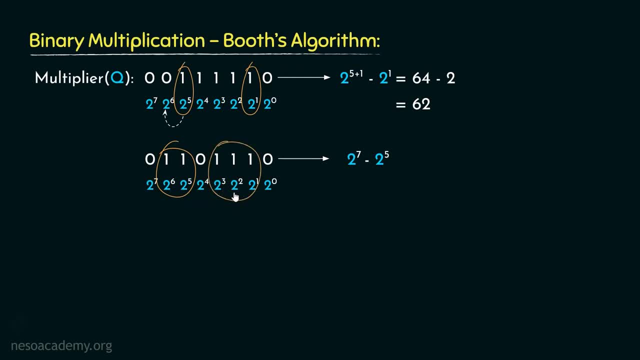 second sequence. observe the bit places: 2 cubed, 2 squared, 2 raised to the power 1.. So the decimal value which we can retrieve from this can be obtained by 2 raised to the power 4 minus 2 raised to the power 1, and once we have determined the values of these, we can obtain the actual value. 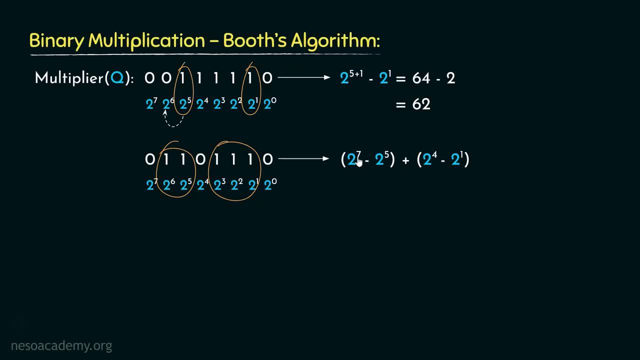 performing an addition. Now, 2 raised to the power 7 is 128, and 2 raised to the power 5 is 32. so 128 minus 32 will give us the result 96.. Now, 2 raised to the power 4 is 16, so 16 minus 2 will give us. 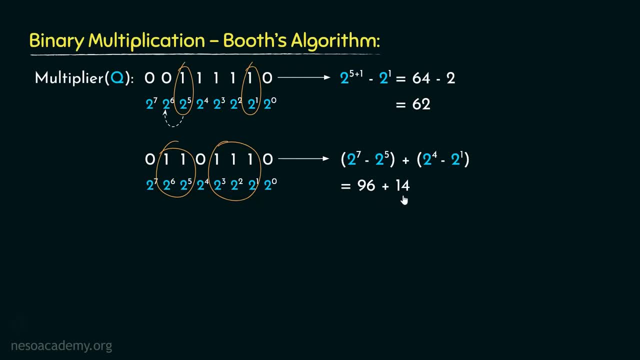 the result 14, and finally, from 96 plus 14 we will obtain the value 110.. So in general, we can state that if we have a sequence like this, which has a sequence of ones in between the sequence and say, the place value of the first one of the sequence is 2 raised to the power j. on the other hand, the 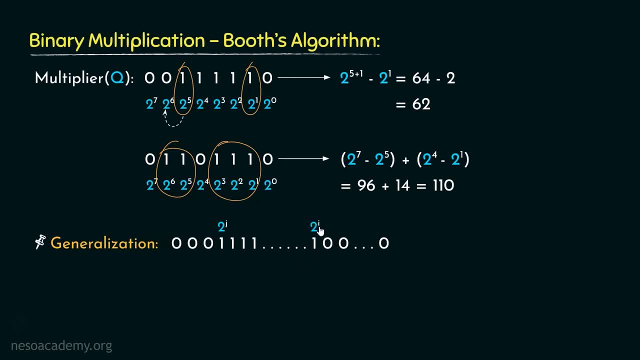 place value of the first one of the sequence is 2 raised to the power j, So we can obtain: the place value of the last one of the sequence is 2 raised to the power i. In that case, these bit sequences of ones will result in the decimal value which can be obtained by 2 raised to the power j. 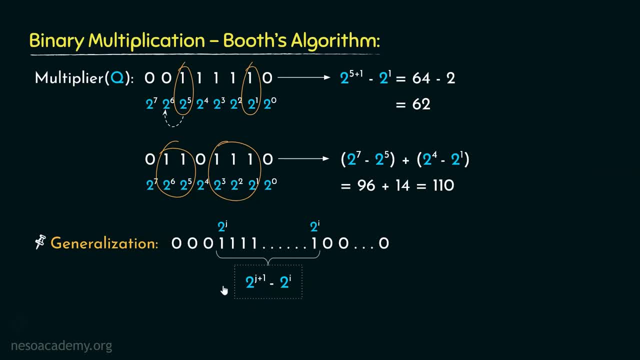 plus 1 minus 2, raised to the power i. Now this one is a very important concept for Booth's algorithm. Now, say we are going to perform a multiplication where we have the multiplicand as 0, 1, 0, 1, 1. 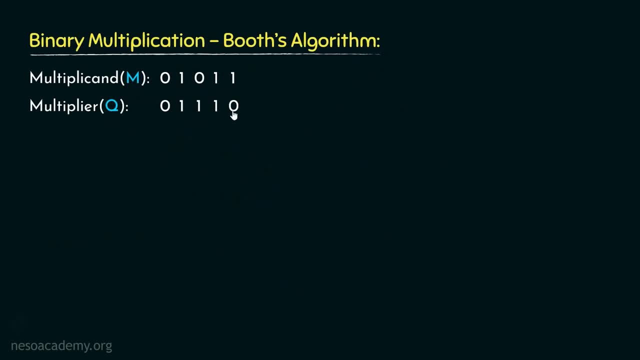 and the multiplier q is 0, 1, 1, 1, 0.. Basically, a sequence of one having a leading 0 and a succeeding 0.. Now observe the place values. So this bit sequence can be decoded as 2 raised to the power 4 minus 2 raised to the power 1.. Now why 2 raised to the power 4? Because 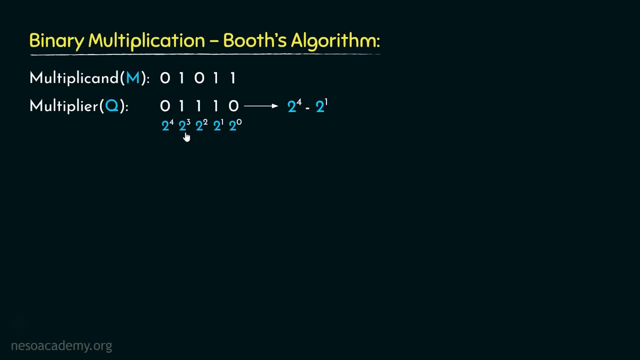 if you observe, the first one in the sequence is placed under the place value, 2 raised to the power 3 or 2 cubed. So we are supposed to have 2 raised to the power 3 plus 1 or 2 raised to the power 4.. 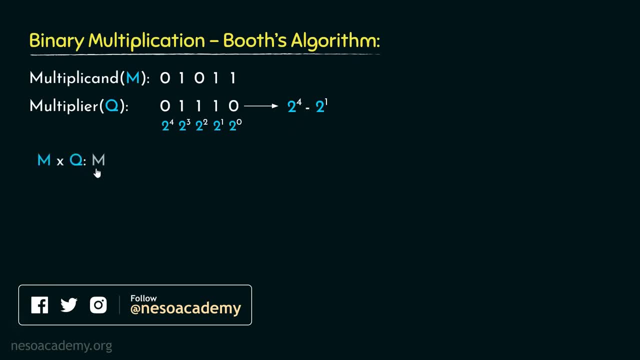 So the multiplication of m and q can be stated as: m multiplied with 2 raised to the power 4, minus 2 raised to the power 1, which is q in here. Now this one can be stated as: 2 raised to the power 4 multiplied with m minus 2 raised to the power 1 multiplied with m. Now in this section, 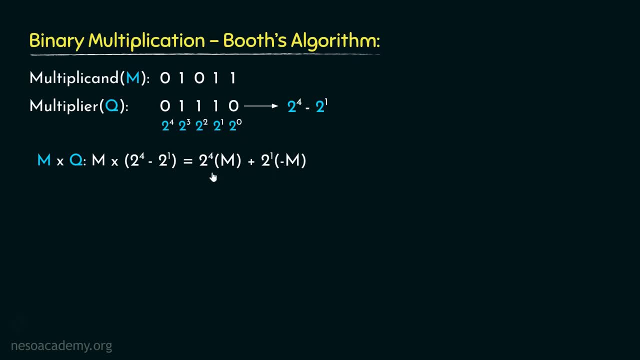 if we push the minus sign inside the bracket, the entire expression becomes an addition. Now, what is minus m? Basically, it is the negative inverse of m. Now, since m is 0, 1, 0, 1, 1, let's determine the negative inverse of m into the negative inverse of m. So we are supposed to have 0, 1 0, 1, 1. 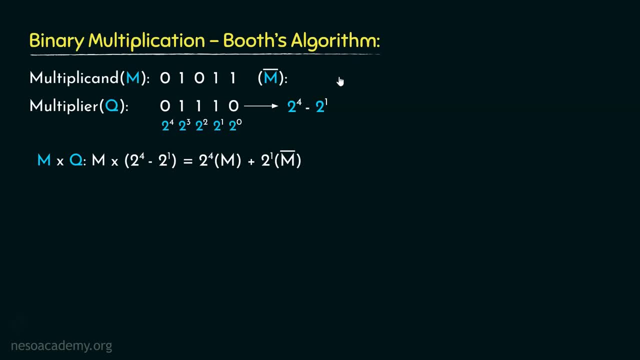 multiplied with m. I believe you remember the process Basically, when we traverse the bits from right to left. if we come across the bit 1, we are going to retain it as it is. thereafter, all the remaining bits are to be toggled like this. So the 2's complement of m is 1 0 1 0, 1.. Let's now 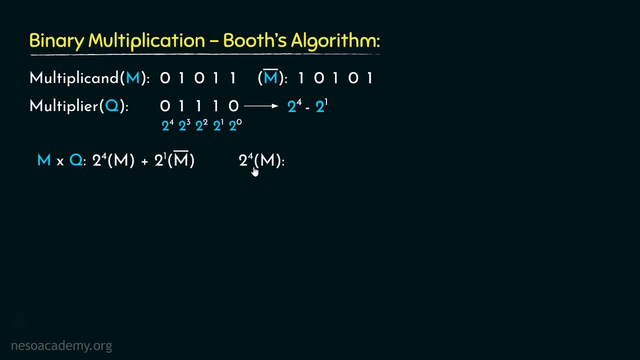 determine this. and this So 2 raised to the power 4 multiplied by m means we will have m first and then multiply it by m. So 2 raised to the power 4 multiplied by m will be the negative inverse of m 2 raised to the power 4.. Now the result of this multiplication will have 4, succeeding zeros by 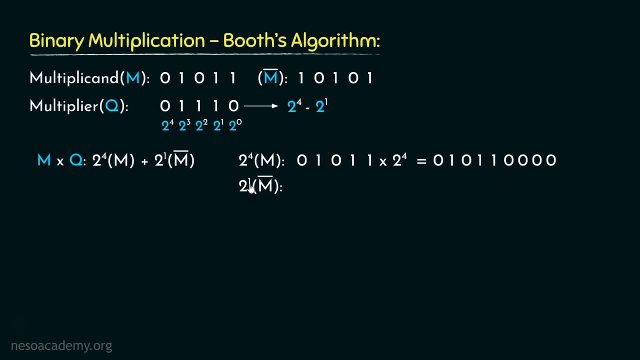 the end of the sequence. Let's now determine 2 raised to the power 1 multiplied with m's negative inverse. So we will have the m complement value in here and multiply 2 raised to the power 1 with it. Now, since the exponent is 1, in the result we are going to have 1, zero at the end of the 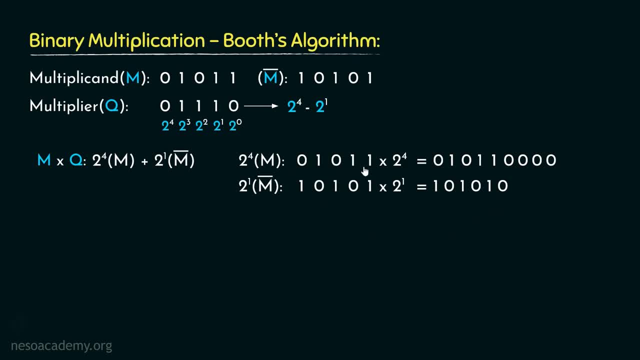 sequence. Now, basically, whenever we multiply a sequence with some power of 2, we are actually shifting the bit sequence towards the left, and that too by the number of zeros, as mentioned in the exponent Observe. we multiplied this bit sequence with 2, raised to the power 4.. So 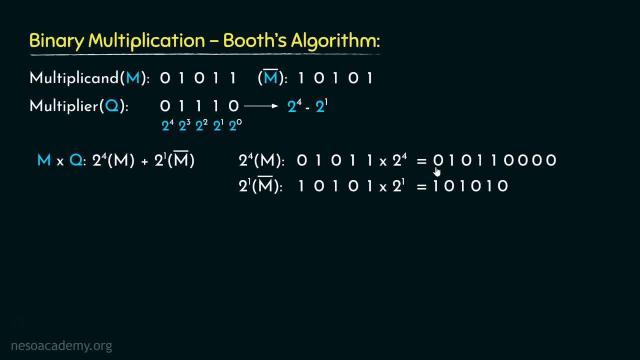 basically, we moved this bit sequence 4 times towards the left. Similarly, when we multiplied this bit sequence with 2, raised to the power 1, we actually shifted this sequence towards the left by 1. and this is pretty evident: When we multiply, we actually shift towards the left, and when we 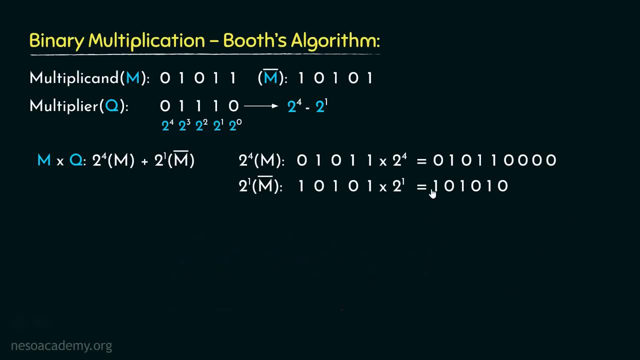 divide, we actually shift towards the right. Now notice carefully. the number of bits in here is 1,, 2,, 3,, 4,, 5,, 6,, 7,, 8 and 9.. On the other hand, in this we have 1,, 2,, 3,, 4,, 5, 6 bits. Now we need 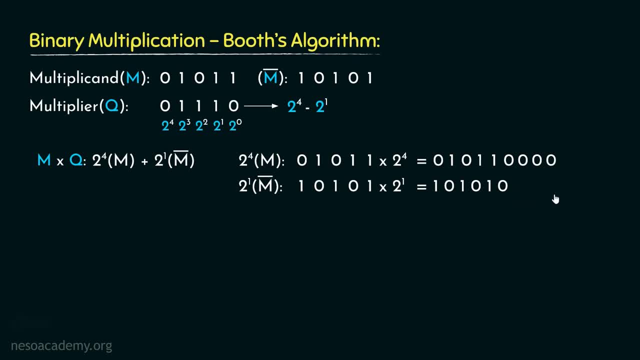 to extend this one to 9 bits. Now, remember, we cannot just extend it, as we can extend the unsigned numbers, because here we are having the negative inverse of m. So how will we extend that? For example, we are supposed to copy the contents at the least significant places first, and thereafter. 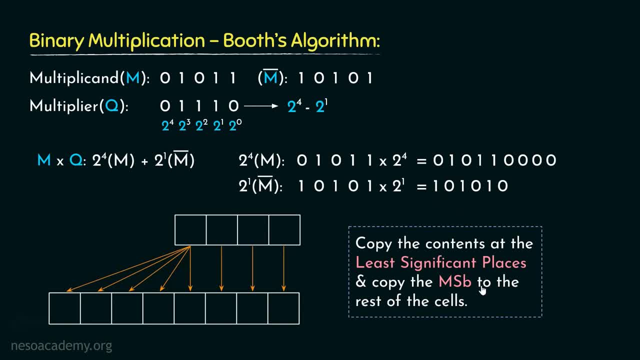 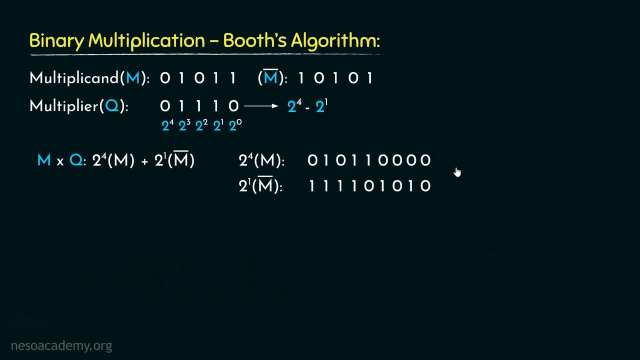 copy the msb- that is the most significant bit of the sequence- to the rest of the cells. So let's perform that. So we are going to copy this entirely towards the least significant places, right, And this is the msb. So we will copy that in the remaining bit places. Now, both of them are. 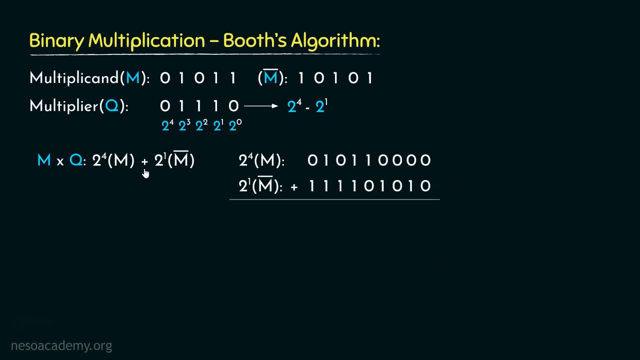 of equal bits. So now we can perform the addition. Let's proceed with the addition now. 0 plus 0 will be equal to 0.. So now we can perform the addition. Let's proceed with the addition now. 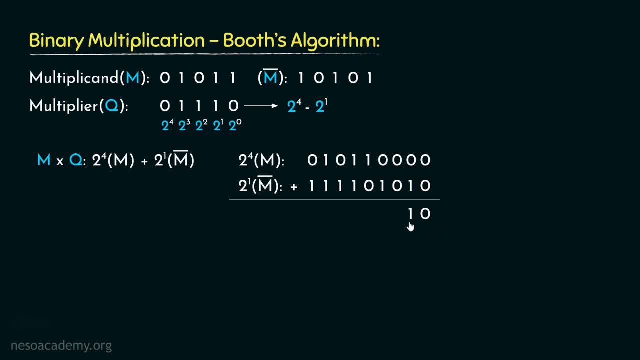 0 plus 1 will give us 0.. 0 plus 1 will give us 1. only Then again we will obtain 0 in here and 1 in this place. Thereafter, 1 plus 0 will give us 1.. Now, 1 plus 1 is actually 1, 0. So we will have. 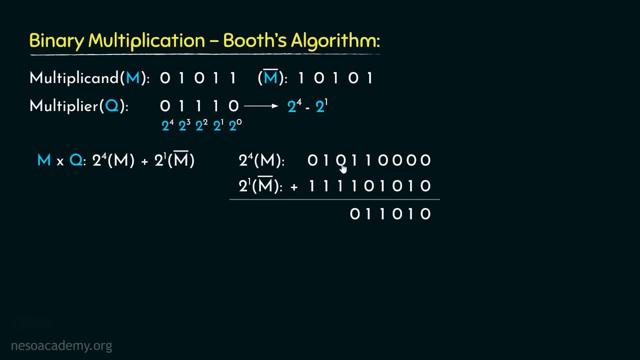 0 as sum. Now the carry one will be added with this 0, making it 1.. So 1 plus 1 will again give us 1, 0.. So 0 we will get as sum, And now that 1 will be added with this 1.. So 1 plus 1, 1, 0.